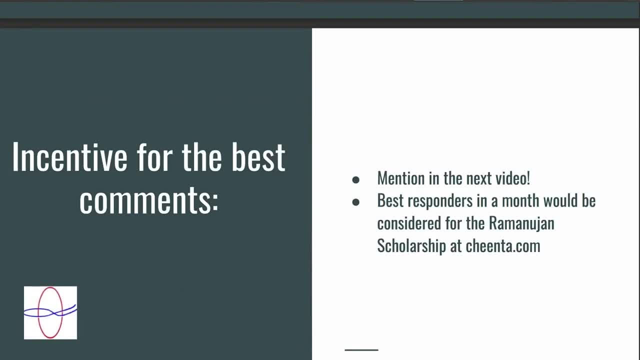 We would like the best comments on this video as responses in general or as solutions to the challenge problem. The best solutions and the best comments will receive either a mention in the next video And the best responders over a month will be considered for the Ramanujan Scholarship at chingtacom. 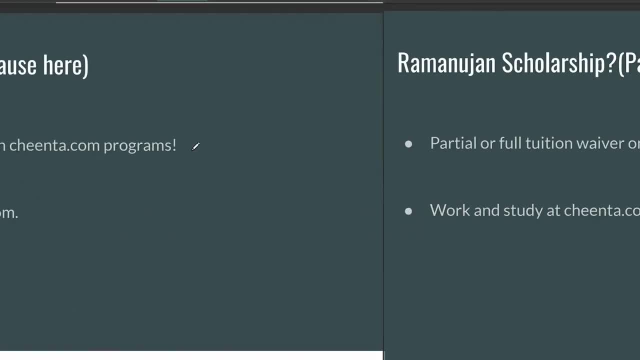 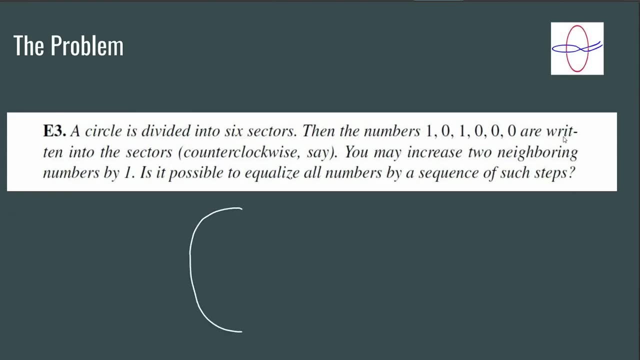 To read more about the Ramanujan Scholarship, feel free. The problem is that we have a circle. We have a circle- Sorry for the drawing- And we've divided it into six sectors. We've divided it into six sectors. We've written the numbers 1, 0, 1, 0, 0, 0 in a counterclockwise fashion. 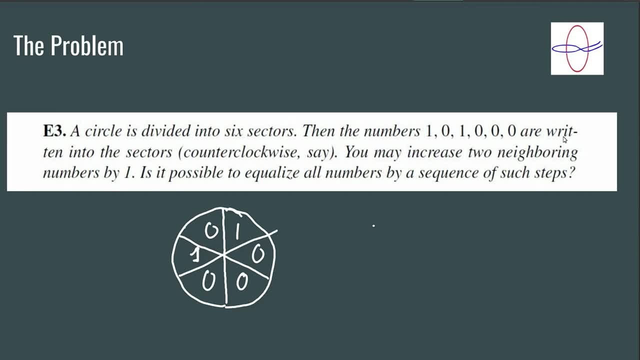 It doesn't really matter if you do it in a clockwise or a counterclockwise fashion, But let's go with counterclockwise. What we are allowed to do is: we can take. We can take two neighboring sectors and increase the numbers in them by one at the same time. 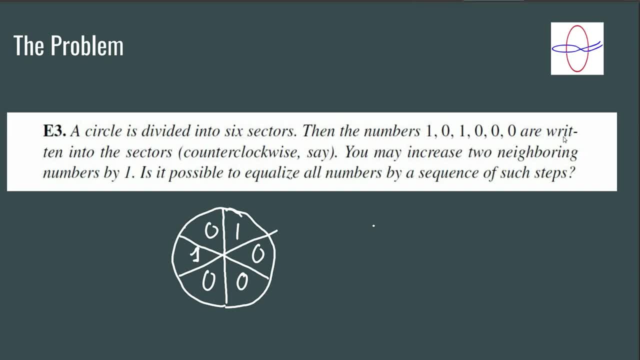 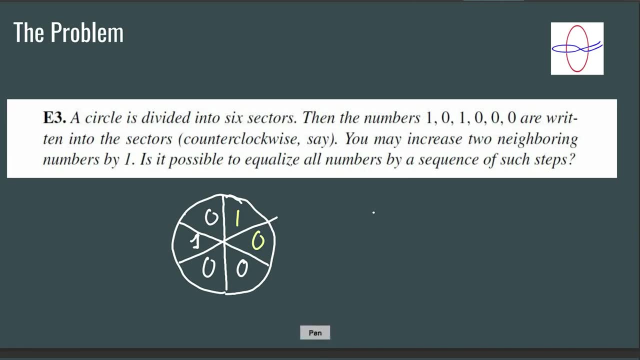 So we can say: take these two sectors, Say we can take these two sectors and increase them both by one. We can do a plus one here and a plus one here to get a new setting. You can change the system to get 2, 1.. 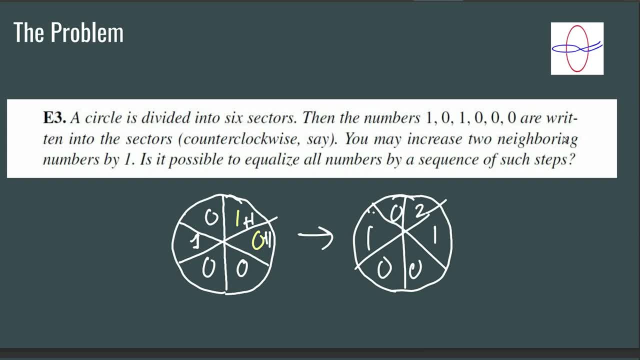 1, 0, 0, 1, 0.. This is what one step of a process could look like. The answer that we're trying to find is: is it possible to equalize all the numbers by a sequence of such steps? 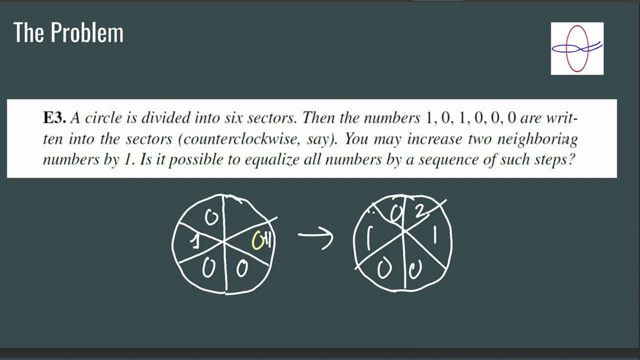 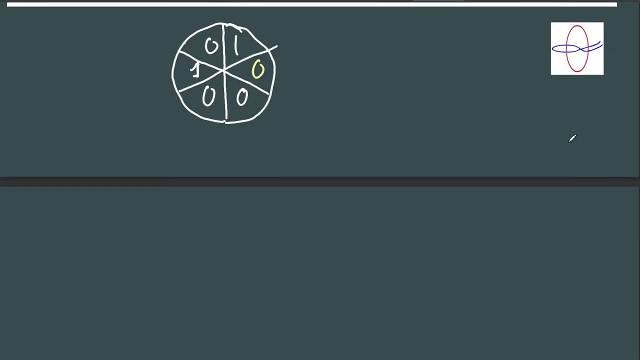 So you start with this setting And we do this process Until we get all numbers to be equal. Now, is this a possible scenario? This is the question we're trying to answer Now. I would just like to take a few moments to discuss what the invariance principle even is, and how is it helpful. 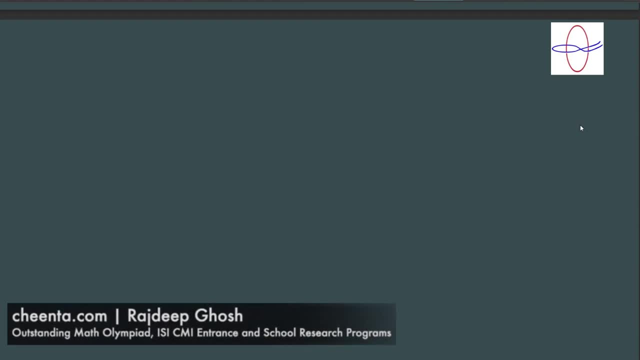 You have a certain process. So say you have a certain object, We'll call it T, And there is a change happening to the process, So it goes from say T0 to T1.. There's a process that's happening. 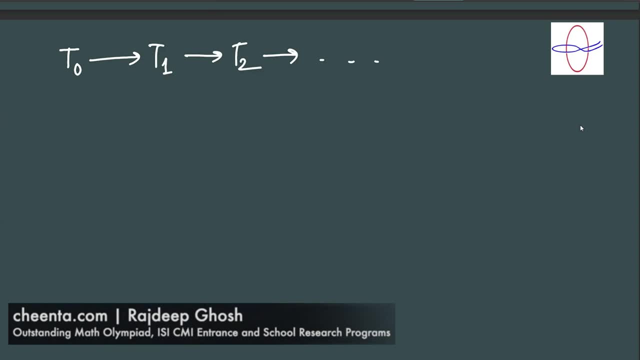 This is your. This process is happening. These are all states of your object. Now you want to make comments about all the future states. So say you want to make comments about T5 and up. We want to make some comments about this. 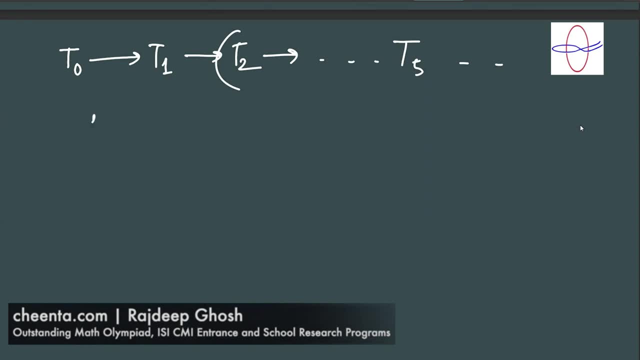 So what the usual idea is? we want to find a function of the state. This is a little bit of formalism, but it's slightly helpful than just throwing around words. We define a function on the state Such that F of T0 is equal to F of T1.. 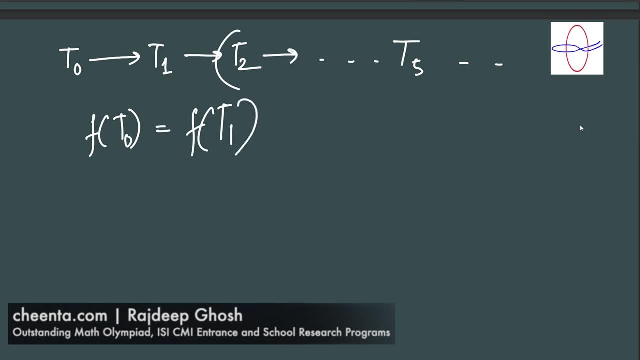 And because the change is the same, we are applying the same change over and over again. So the change that happens between T0 and T1 is the same change that happens between T1 and T2.. This keeps on happening. So the function F is what we call an invariant of the state. 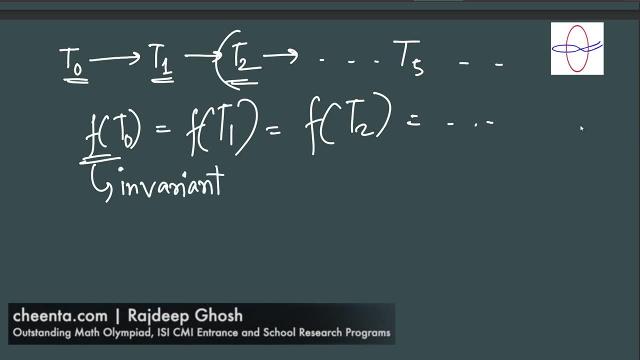 It is a quantity that stays the same throughout the process. Now do you see how that is helpful? So you know if something, If the value of this quantity is something at the beginning, if F of T0 is something C- and this is known to us- F of Tn is equal to C for all n. 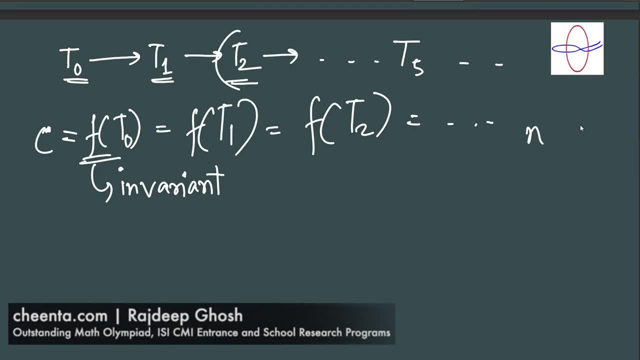 So this is extremely helpful. We can make comments about the property F of all the future states. Now, this is a lot of formalism And in fact, this is what we call a heuristic principle. The invariance principle is what we call a heuristic principle. 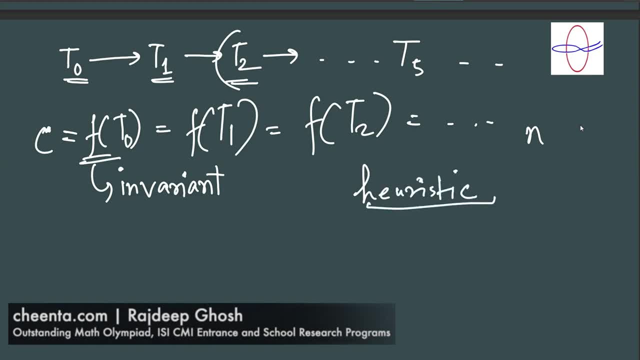 It's just a fancy word, Which means that it's the kind of principle where there is no big central theory. It's the kind of thing that you can learn only through problems, So there is not much theory to it, It's mostly problem solving. 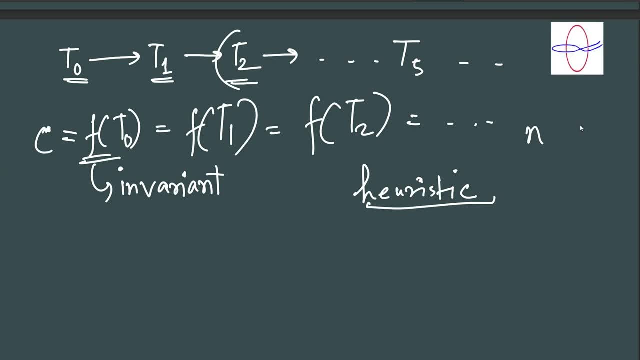 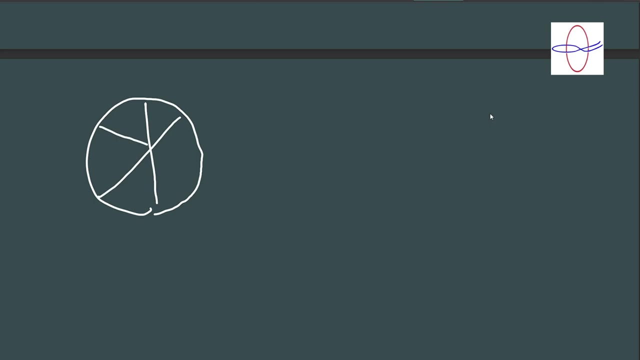 And you get more and more well-versed with the theory simply by doing more problems. So coming to the problem. So obviously the idea is to construct an invariant. We would like to take our setup. The numbers themselves are irrelevant Because the process 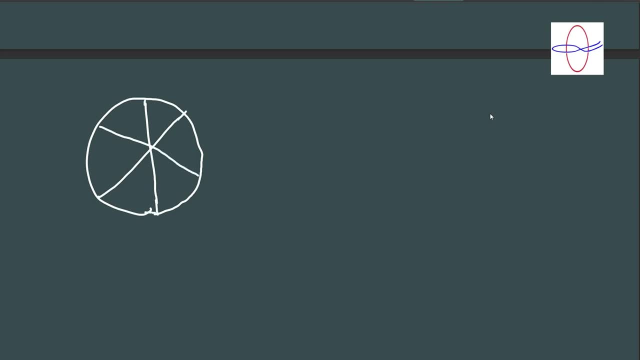 Well, they are relevant, obviously, But you could shift them all by the same quantity and they would be the same Point is that if I have A1, A2, A3, A4, A5, and A6., 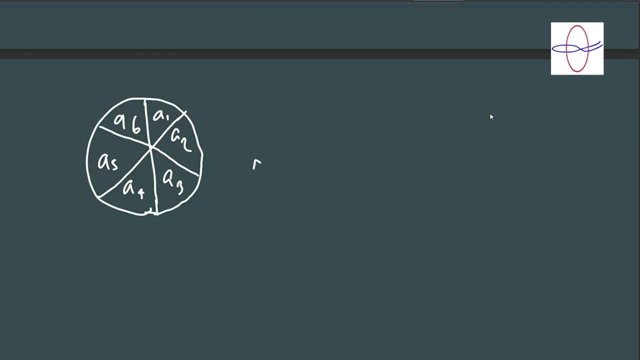 We would like to find an invariant with this state. So the state could. The circles in the sectors are slightly. They set you off a little bit. The point is that you can take any two consecutive ones, And A6 and A1.. 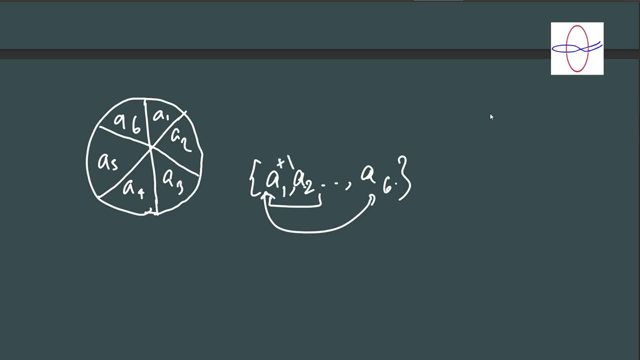 Are considered consecutive And you can increase both of them by one, Or something like this. This is what the state is. You would like to form An invariant is not immediately visible, So you would like to construct an invariant with some cleverness. 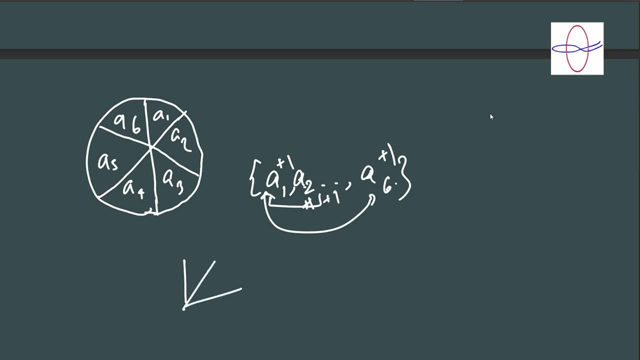 Clearly, what's happening is we take two adjacent sectors, Consecutive sectors, And we increase them both by one. Doesn't it make sense to just consider A1 minus A2? Right, So if we consider A1 minus A2, since they're both increasing by one, there is no net change. 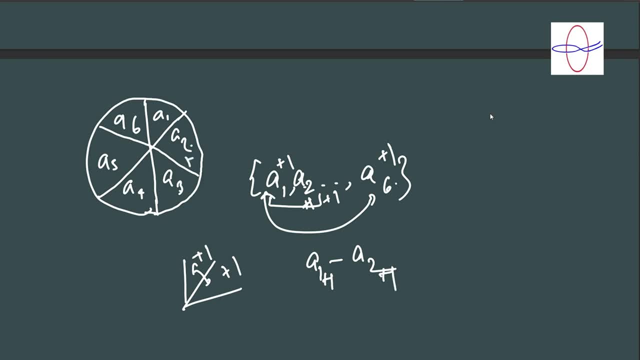 The thing is, you could also have increased A2 and A3. Well, in that case we could need something like A3 minus A2 or A2 minus A3. In this case, we could have A2 minus A1 or A1 minus A2.. 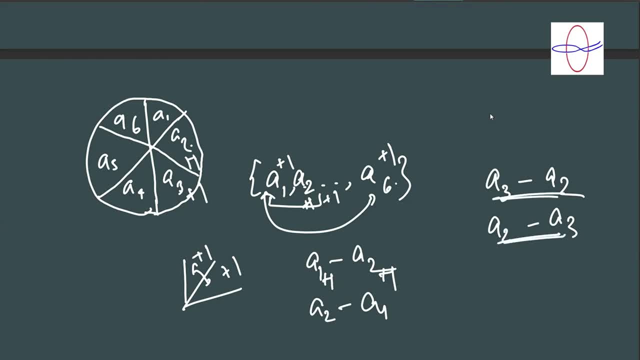 Either of these works And these values stay the same. The thing is, we don't really know which two numbers we'll pick, So we'll have to construct an invariant. It stays the same no matter what move you make. So, with some cleverness, and noticing that A1 minus A2.. 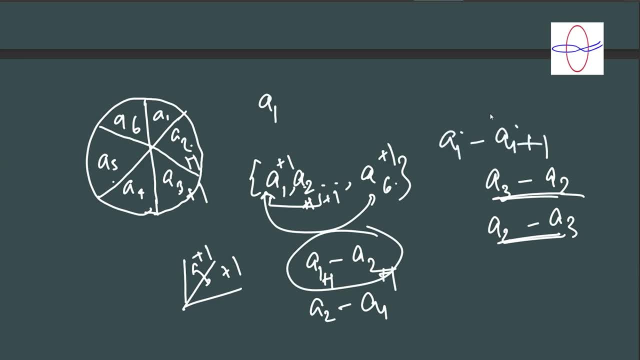 AI minus AI plus 1 stays the same. If you, you know, fix a. If you, you know, take the sectors AI and AI plus 1, and you increase them both, the difference stays the same. If I consider this number, 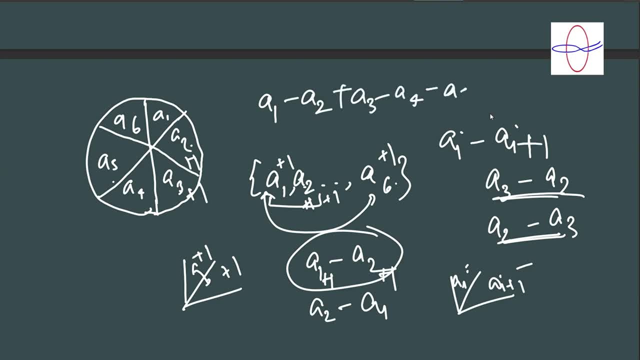 We have A1 minus A2, A3 minus A2, A3 minus A4, A5 minus A4, and A5 minus A6, and A6 minus A1.. 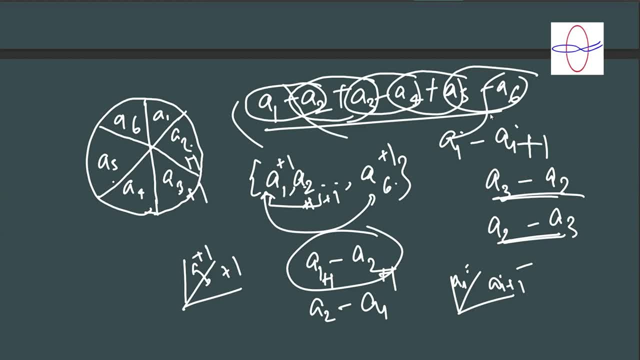 So no matter which two consecutive numbers you pick, since any two consecutive numbers have opposite signs, increasing both of them will not result in any change. So we found our invariant. So our invariant, i you can call it, is A1 minus A2.. 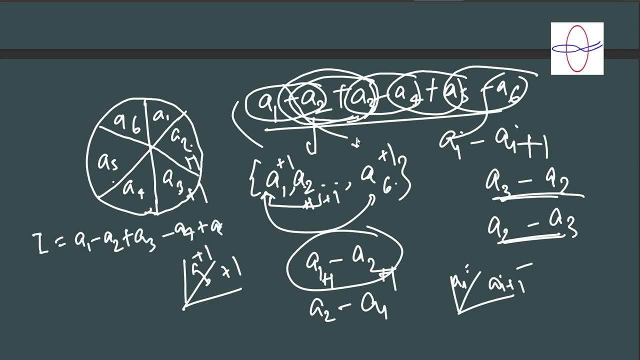 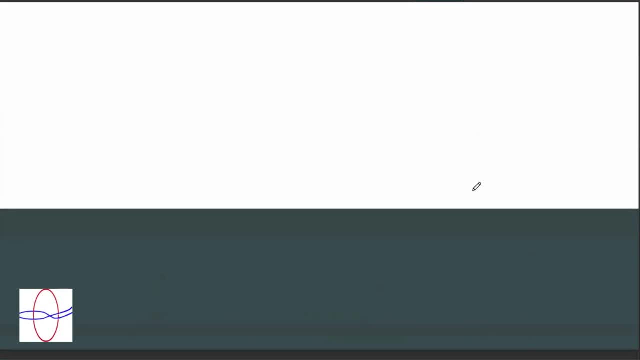 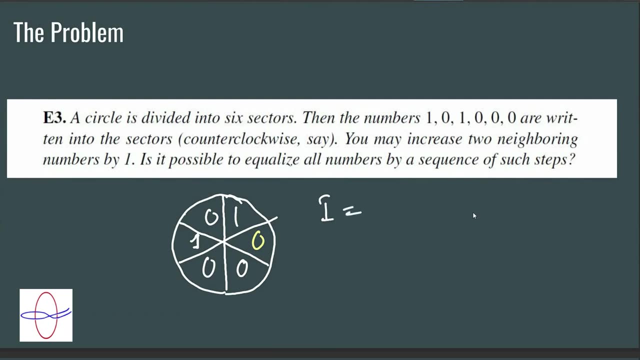 Plus A3, minus A4 plus A5.. So, no matter what moves you make, the value of A1 minus this value has to stay the same. Note and well, we can see this as an example. If we start off like this: what is our initial, what is the value initially of i in our initial configuration? 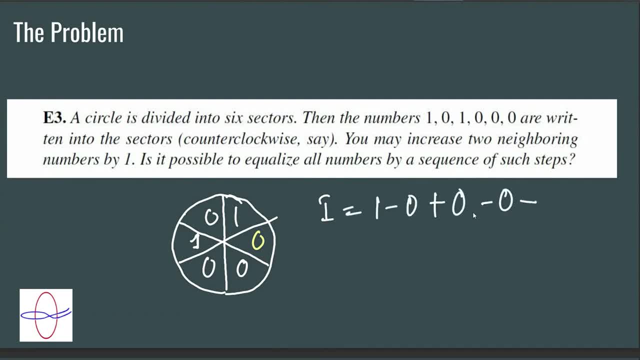 It's 1 minus 0 plus 0 minus 0 plus 1 minus 0.. Initially it's 2.. Right, And just as an example, if we increase this, If we increase these two, what happens is this becomes plus 1, this becomes plus 1, so we have 2 minus 1, but this is still 1, and there's a 1 here, so the value is still 2.. 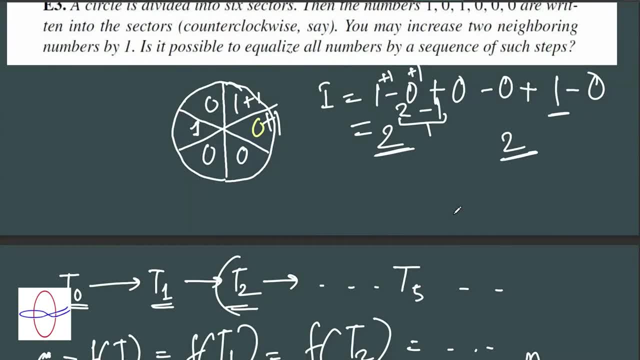 So do you see what's happening? The value stays the same. So initially, the value is 2.. What would happen if, say, it was possible to get to a state where every single number was the same? In that case, isn't the value of this function, you know, A1 minus A2, and so on? doesn't this become 0?? 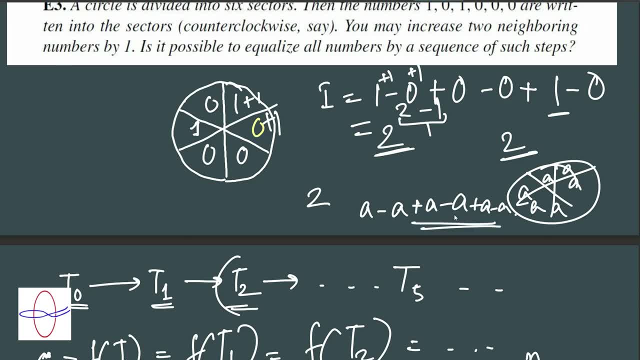 So this, This end state is not possible. You cannot achieve this state simply by virtue of the fact that the invariant has to always be 2. It cannot be 0. So the answer to this question is no, And we're done. 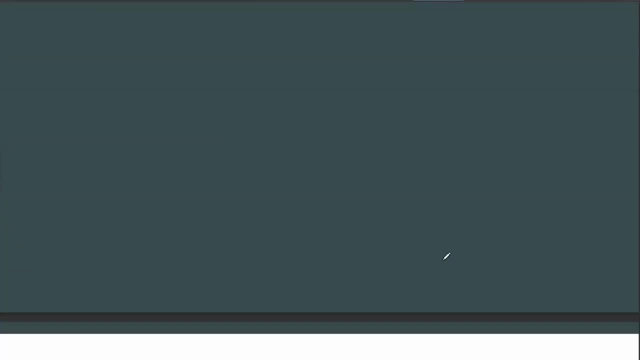 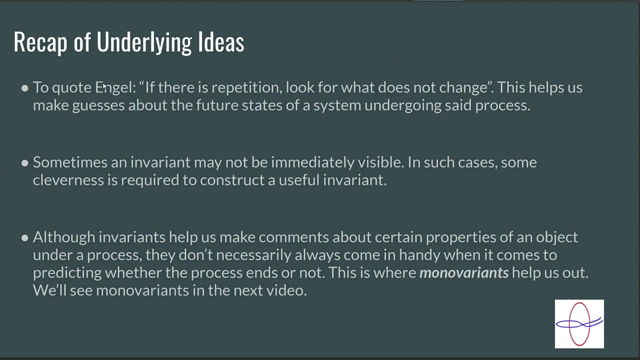 This is the problem And I hope I've made this idea clear. To quote Engel, this is directly from Engel. if there is repetition, look for what does not change. This helps us make guesses about the future states of a system undergoing said process. 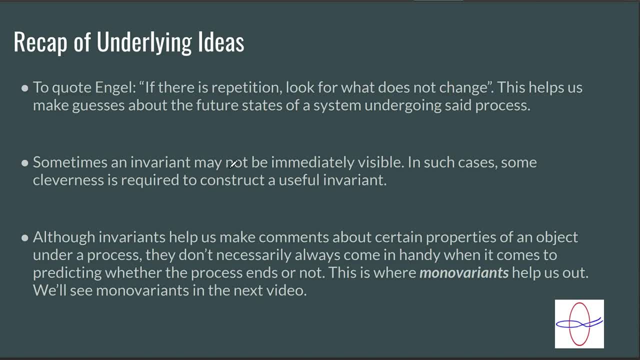 which is what we did here. We constructed an invariant which stayed the same, and hence we could make predictions about all the future states, not just one. We know that the This- you know, all the sectors cannot have the same value, simply because the invariant will not allow it. 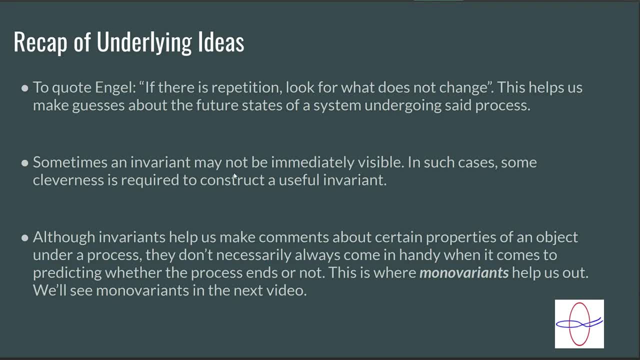 Sometimes an invariant may not be immediately visible. In such cases, some cleverness is required to construct a useful invariant. Now you might find invariants, but they might not necessarily be useful. You need Sometimes you might need some cleverness to come up with an invariant.